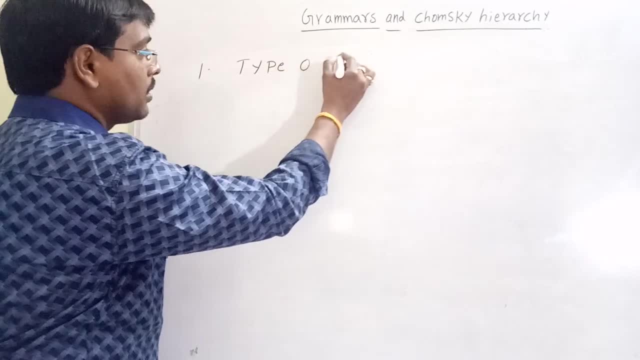 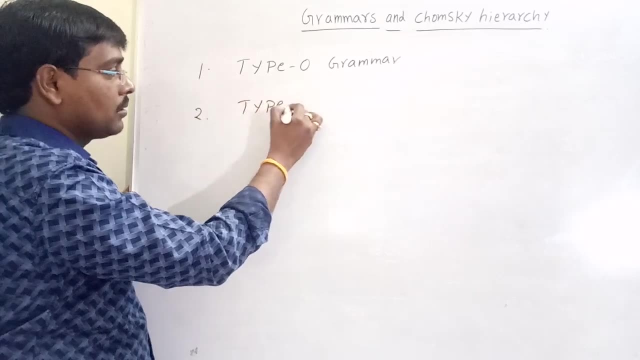 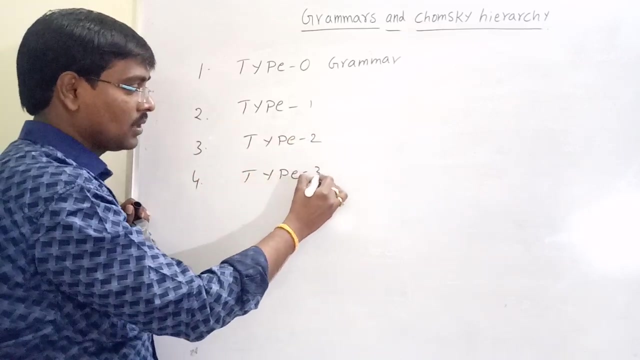 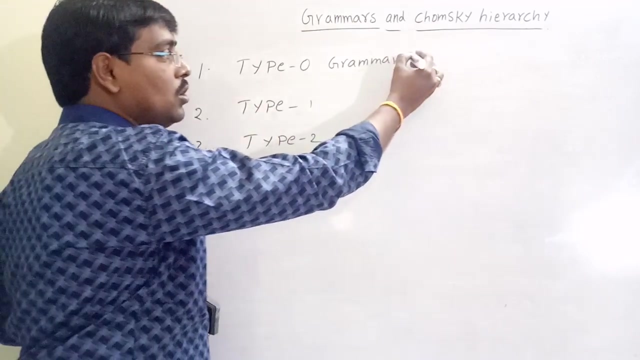 Type 0 grammar. Type 0 grammar, Type 1, Type 2 and Type 3.. These are the four types of grammars: Type 0, Type 1, Type 2 and Type 3.. This Type 01 grammar is called unrestricted grammar. 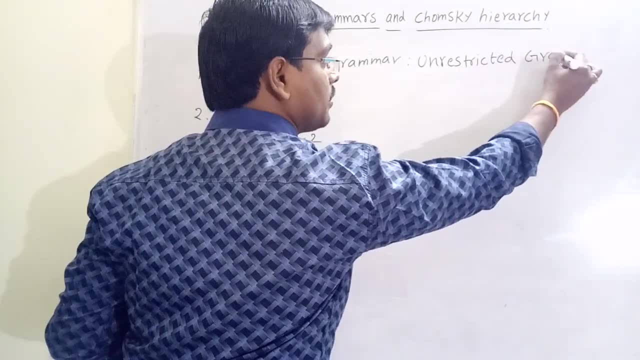 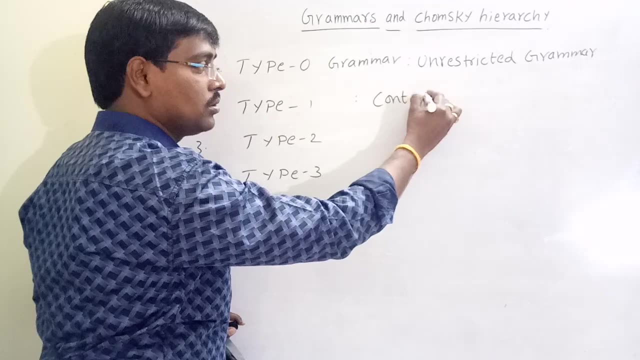 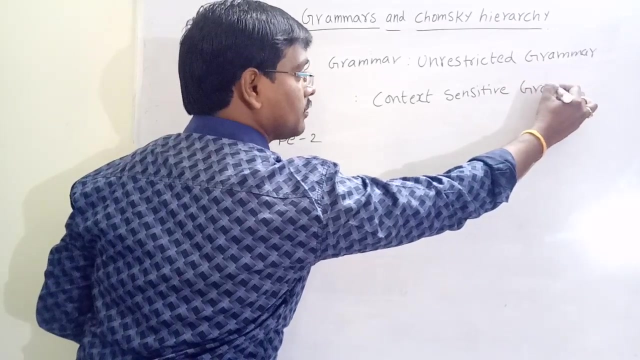 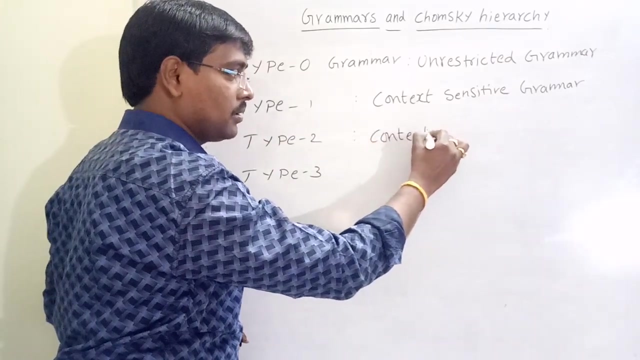 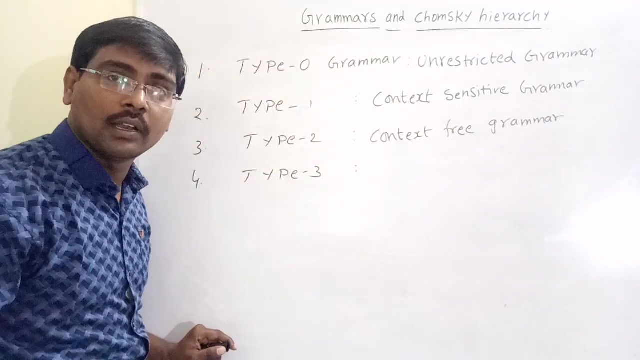 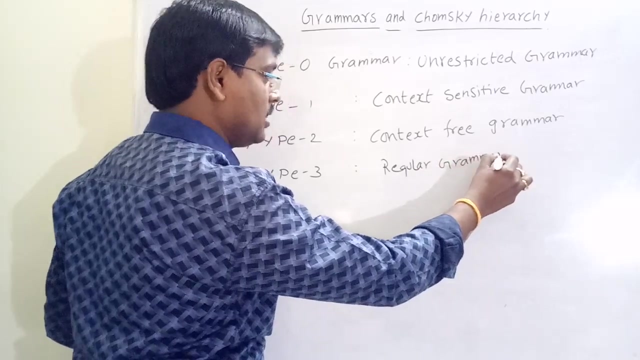 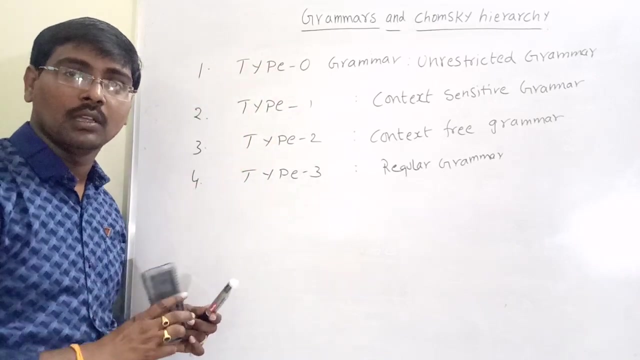 This. Type 01 grammar is called unrestricted grammar. Type 01 grammar is called as context-sensitive. context-sensitive grammar. Type 02 grammar is called as context-free grammar And type 3 grammar is called as regular grammar. These are the classification of grammars. We have four types of grammars: Type 0, type 1, type 2, type 3.. Now, step by step, we will discuss each type of the grammar. 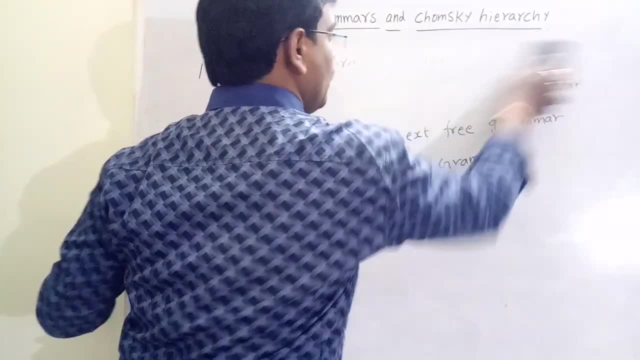 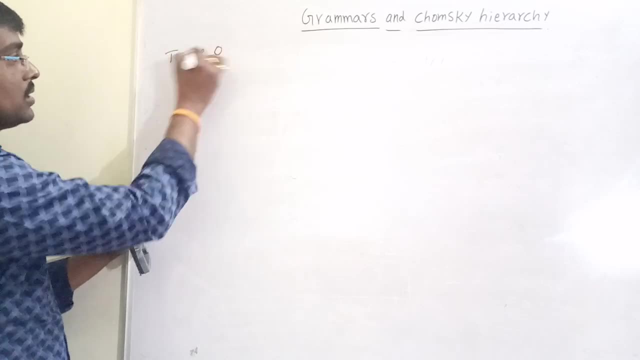 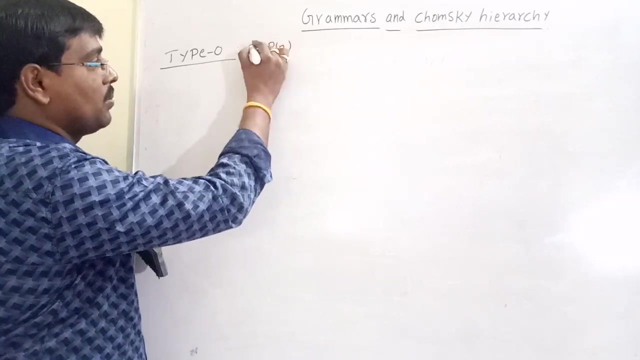 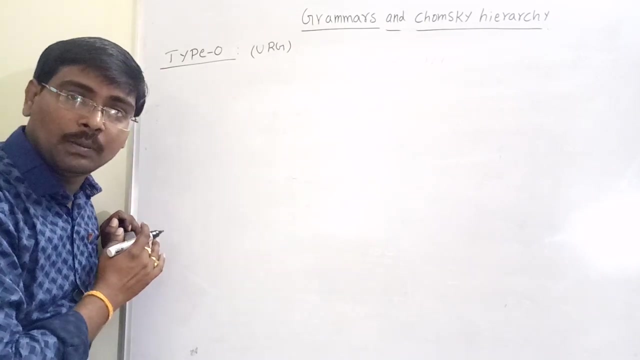 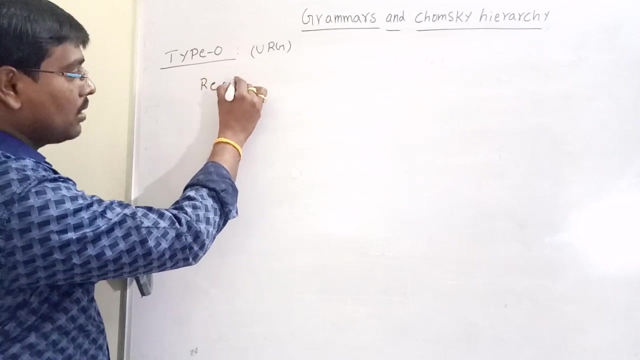 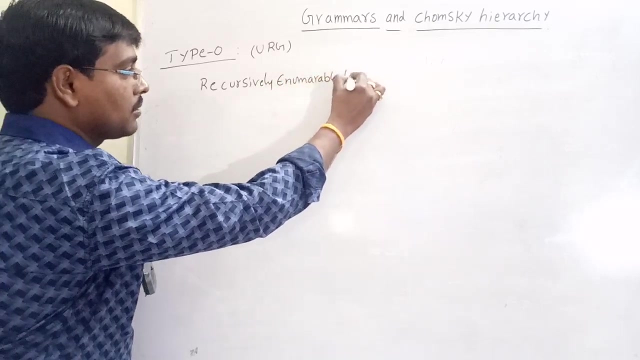 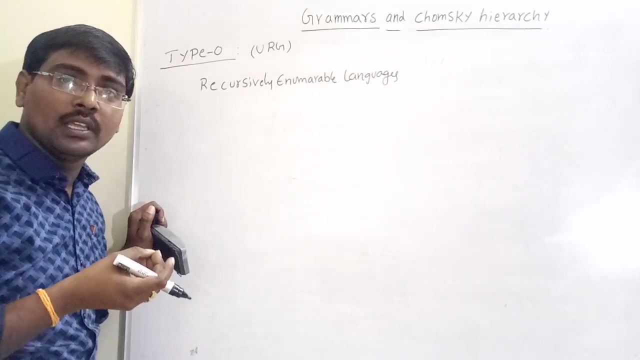 Now, first we will go to type 0 grammar. So type 0 grammar is also called as unrestricted grammar. Suppose these grammars accept all the formal languages, The languages accepted by these type 0 grammar are the formal languages. Type 0 grammar are recursively enumerable languages. Type 0 grammar accept recursively enumerable languages. 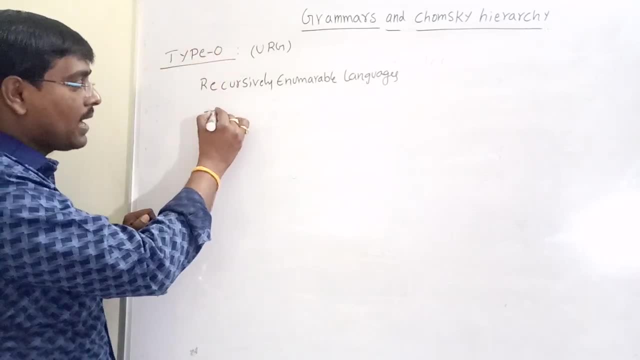 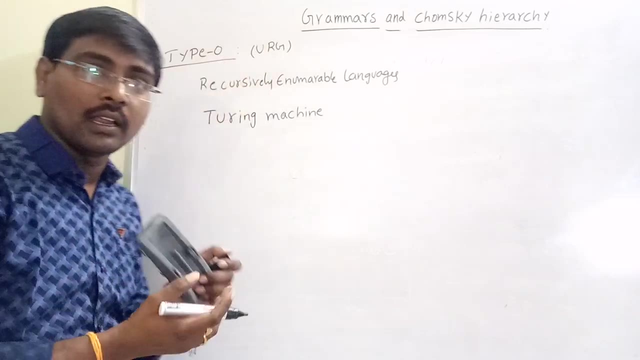 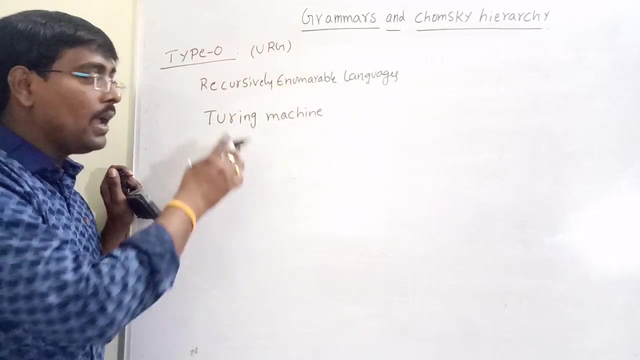 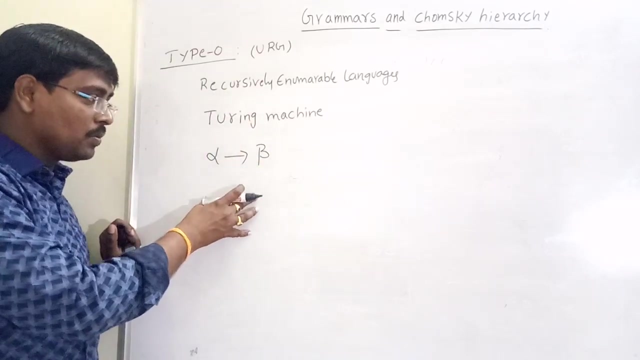 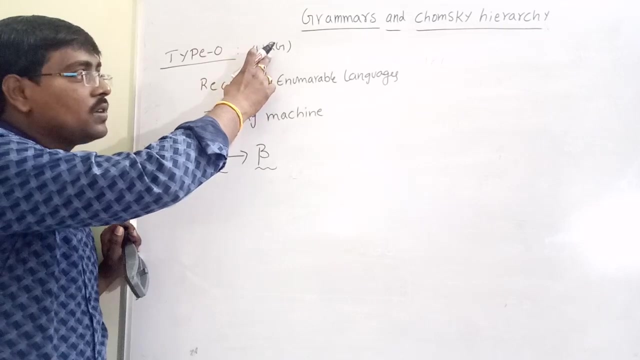 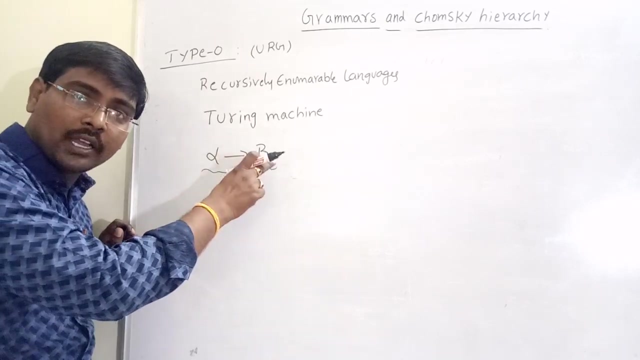 And these recursively enumerable languages are accepted by Turing machine, That is, the grammars are recognized by using Turing machine. This machine generates the recursively enumerable language And each production is of the form alpha tends to beta. Suppose the form alpha tends to beta. Here there is no restriction on alpha and beta. The name itself specifies It is an unrestricted grammar, That is, there is no restriction on alpha and beta. 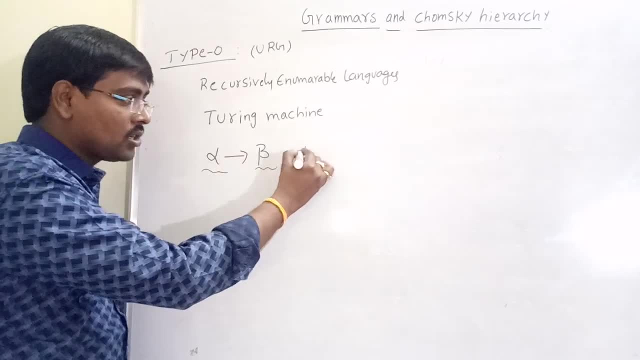 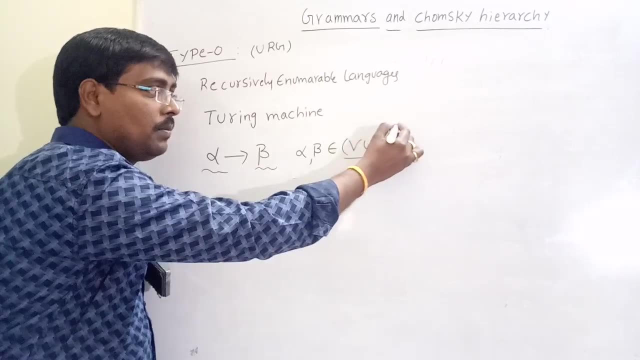 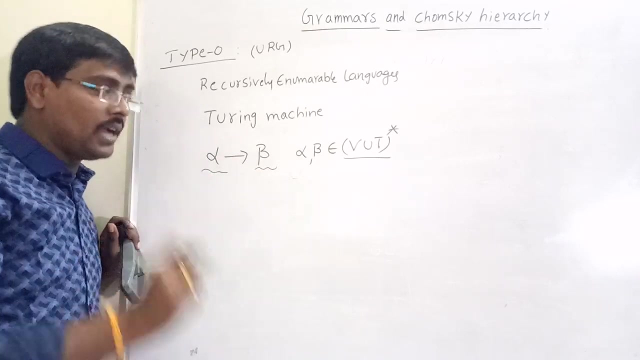 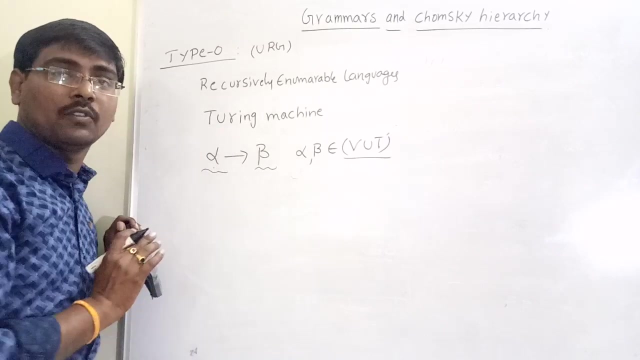 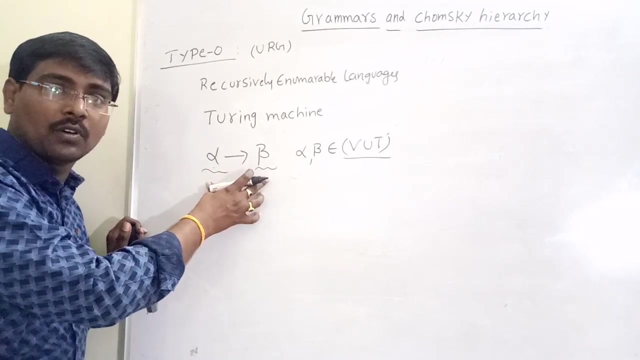 That is, alpha is any combination. Alpha, gamma, beta belongs to V union T, Any combination of terminals and non-terminals. Terminals and non-terminals, But remember, at least one non-terminal is present on the left hand side, At least one non-terminal is present on the left hand side. The production is of the form. 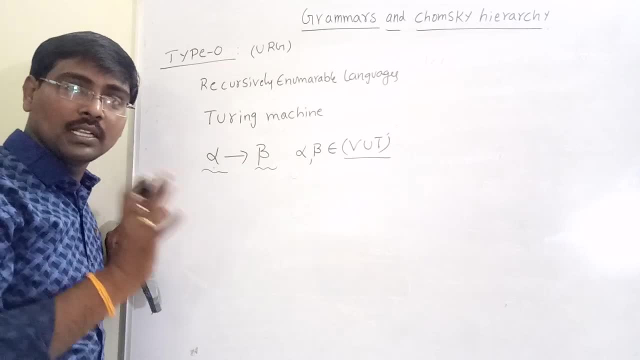 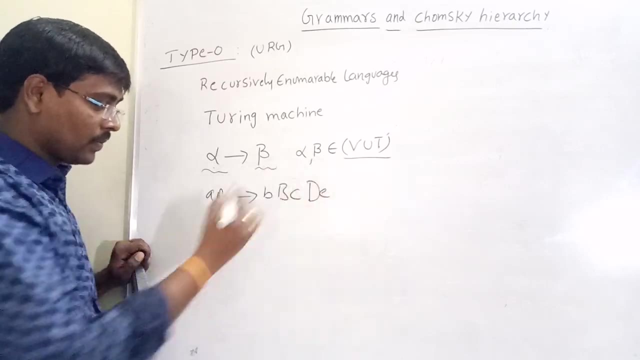 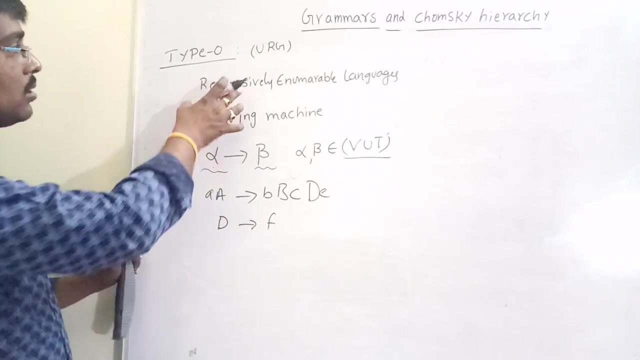 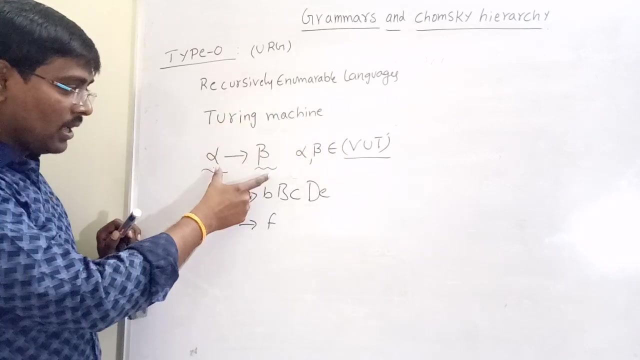 Here there is no restriction on combination Combinations of terminals and non-terminals. For example, A, A tends to B, B, C, D, E, Suppose D tends to F. This is an example of unrestricted grammar. So in type 0, the languages is recursively enumerable language, The automata is the Turing machine. Ending of the form: alpha tends to beta. 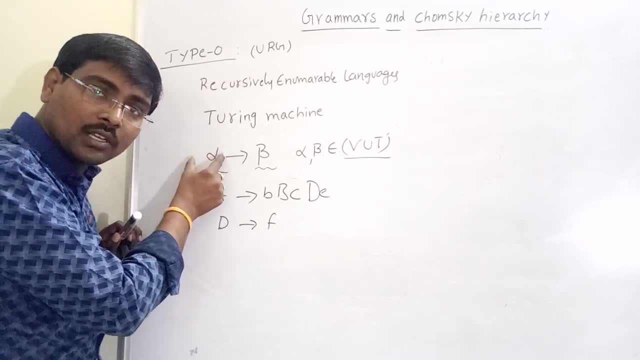 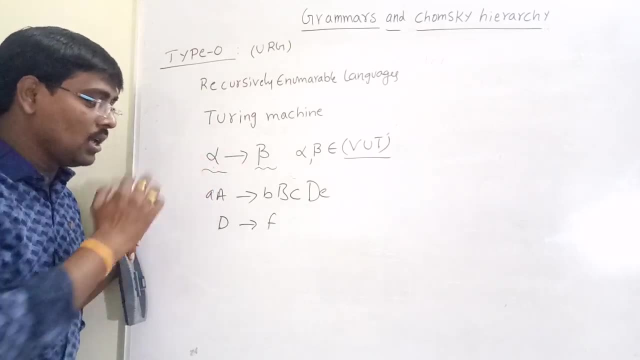 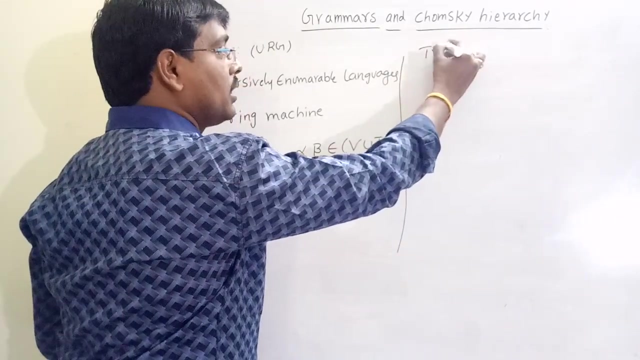 Alpha tends to beta. Here there is no restriction on the combination of alpha, But at least one non-terminal must be present on the left hand side, That is, on alpha. Suppose this is the example Now. type 1 grammar. Type 1 grammar. 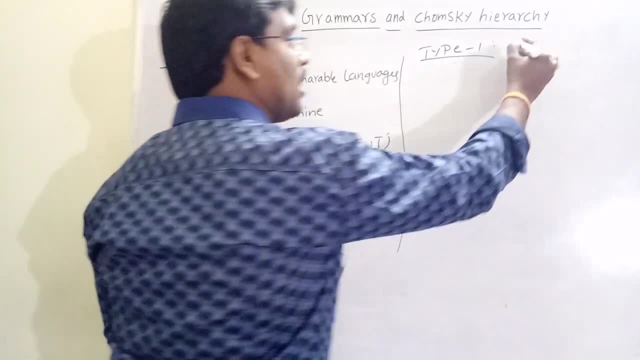 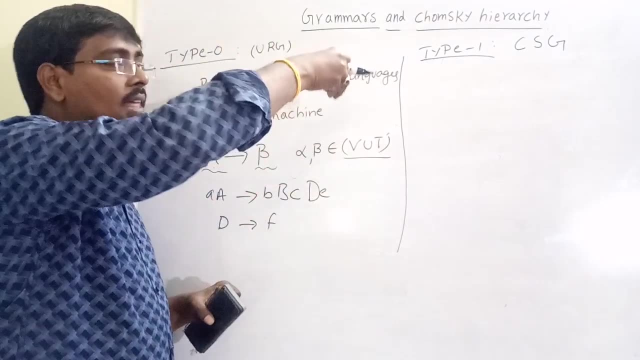 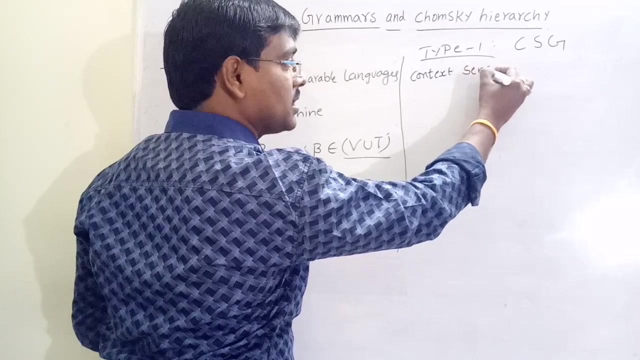 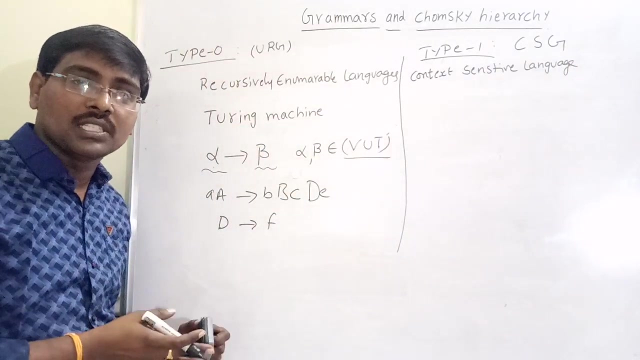 The type 1 grammar is called as context-sensitive grammar. Type 1 grammar is called context-sensitive grammar. The languages generated by this grammar is context-sensitive language. the language generated by this one is the context-sensitive language and the automata that acts as this. 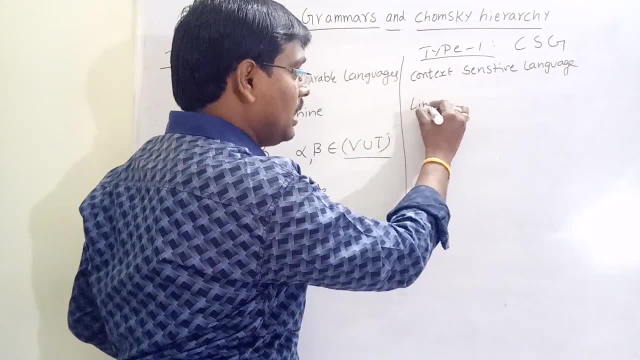 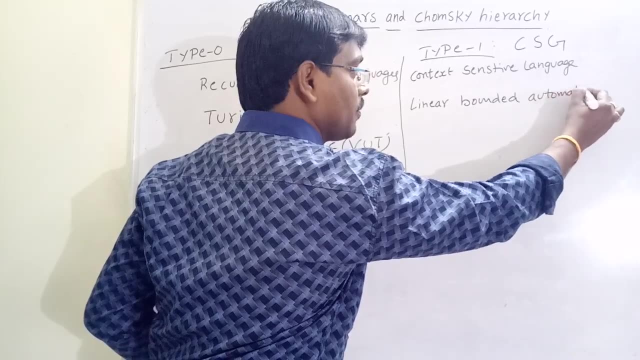 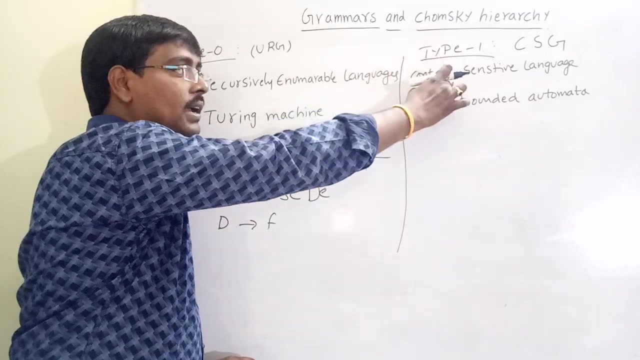 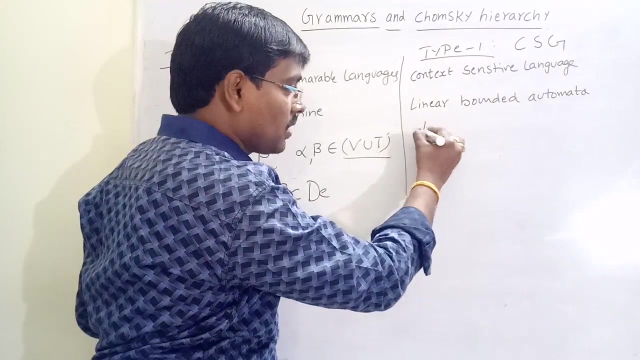 context-sensitive language is linear bounded automata, linear bounded automata, linear bounded automata. this is by using this linear bounded automata, we are accepted the languages, that is, we are accepted the context-sensitive language and the production is of the form. alpha tends to beta, production is 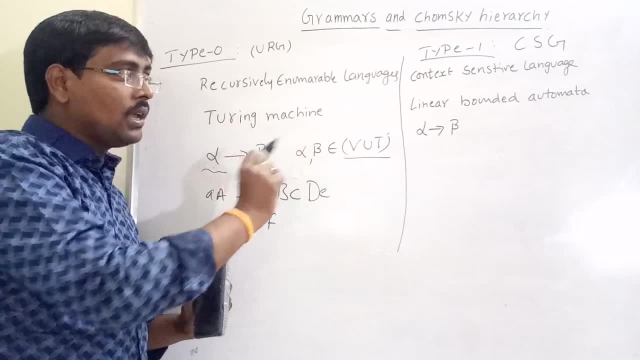 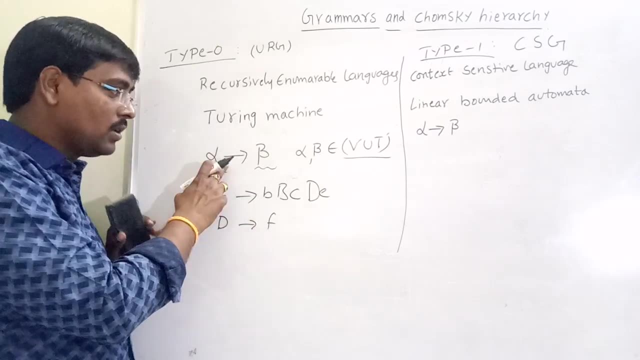 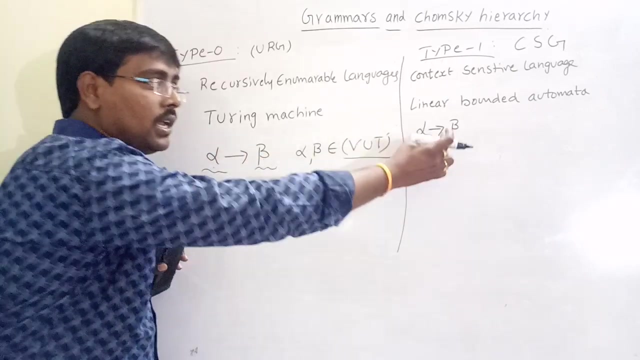 of the form, alpha tends to beta, and alpha and beta is any combinations of terminus and non-terminus similar to the combination of terminus and non-terminus, similar to this one: alpha and beta combinations of either terminus and non-terminus. here also, alpha and beta are combinations of either terminus or 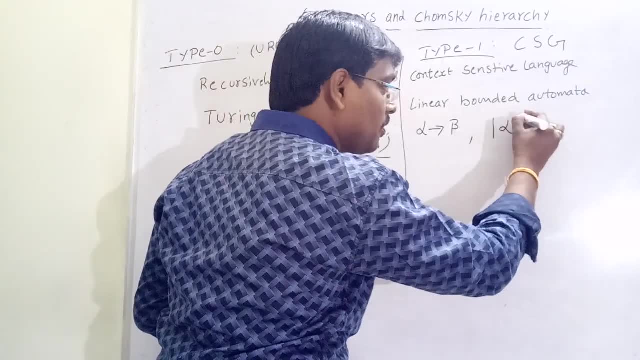 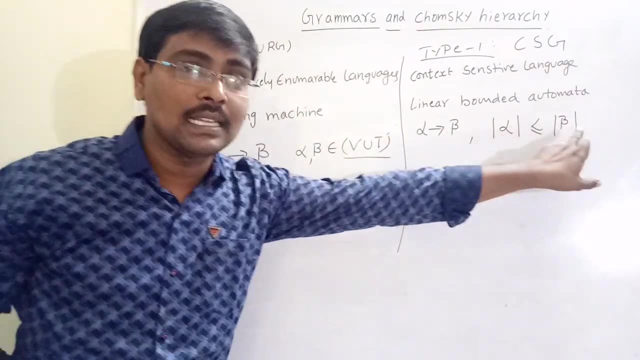 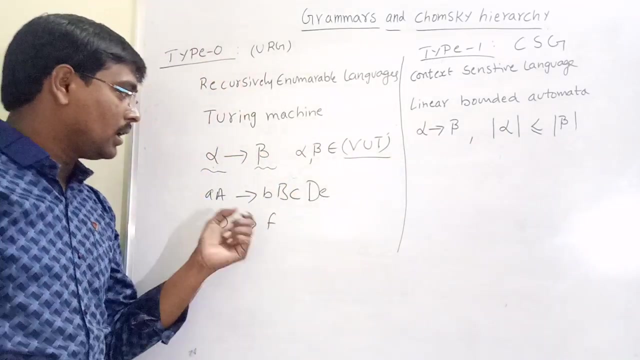 non-terminus, but the length of alpha is less than or equal to length of the beta. the length of alpha is less than or equal to length of the beta and left to hand side compulsory. we have a non-terminus in other cases. left to hand. 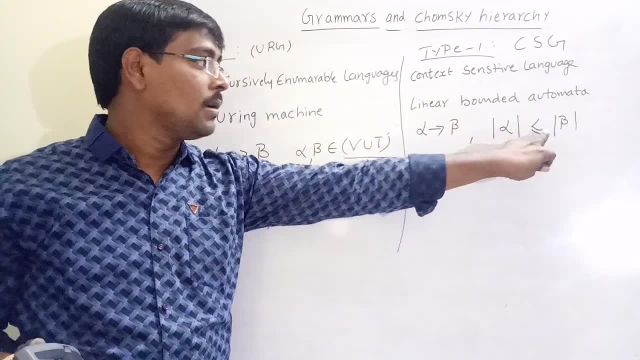 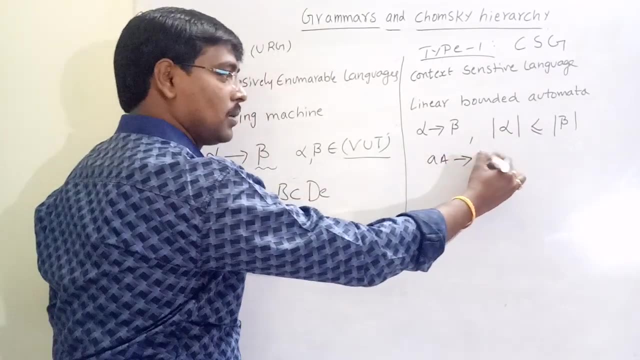 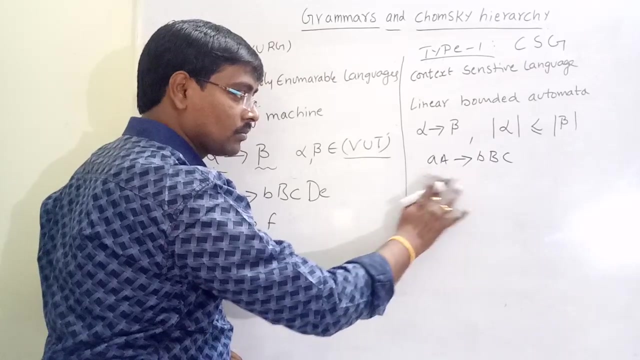 hand compulsory, we have a non-terminus. in other cases, left to hand set we will compulsory and nominal. but here one information is left, fuck saw. here one information is left, fuck saw. here one information is left, fuck saw. let's suppose everything set up on the. 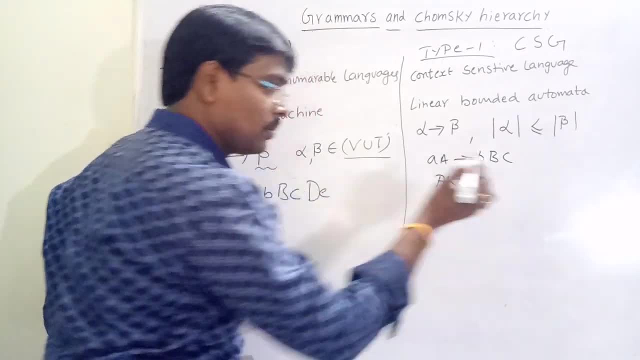 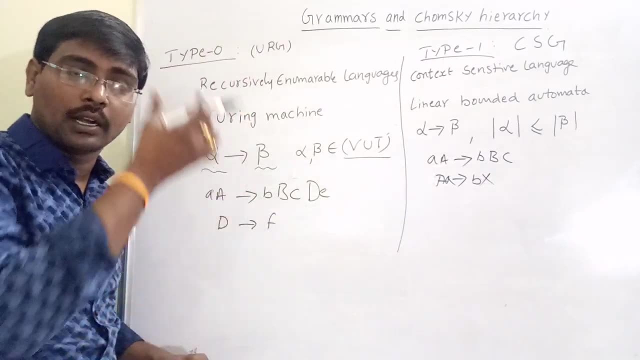 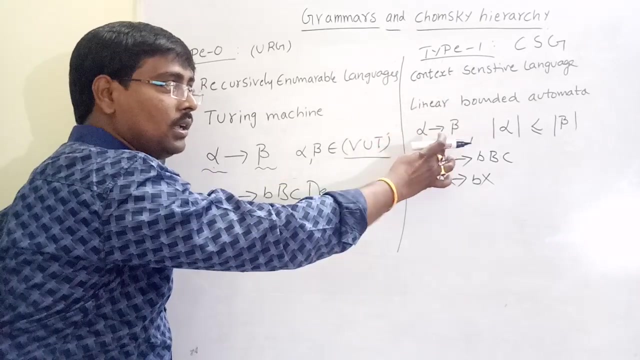 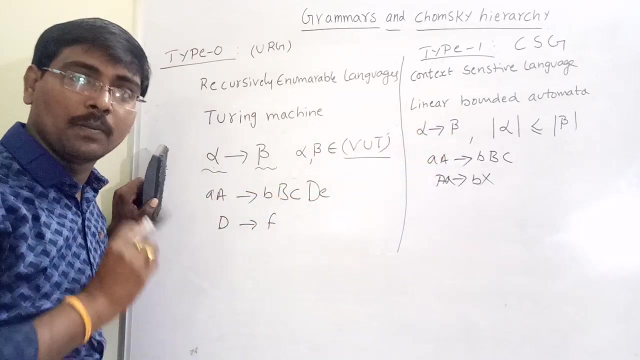 level that we have in the population. This is not accepted. This is not accepted. This is type 1 grammar Context, sensitive language accepted by the linear automata and production is of the form alpha tends to beta, where alpha and beta is a combination of terminals and non-terminals, but the length of the alpha is always less than or equal to beta. 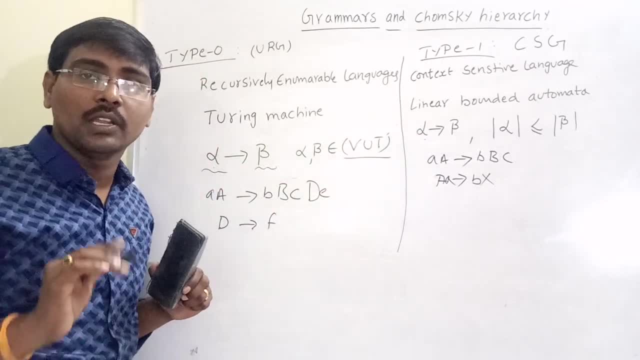 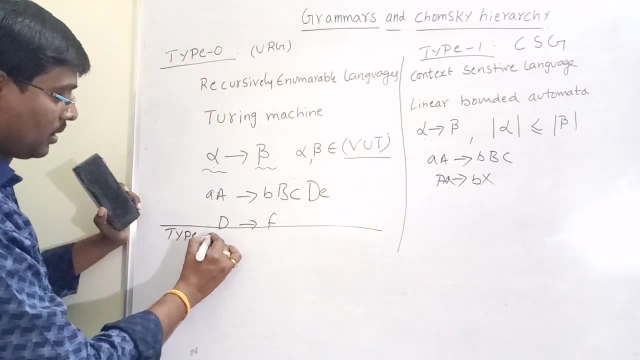 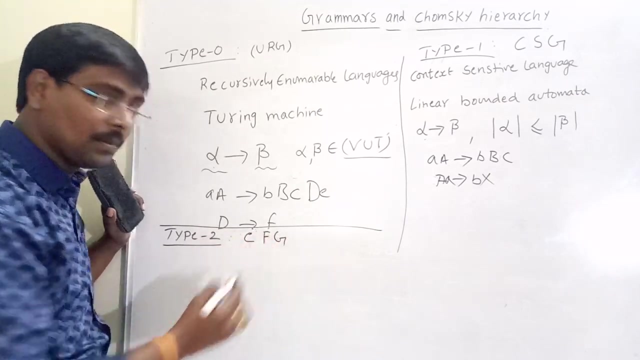 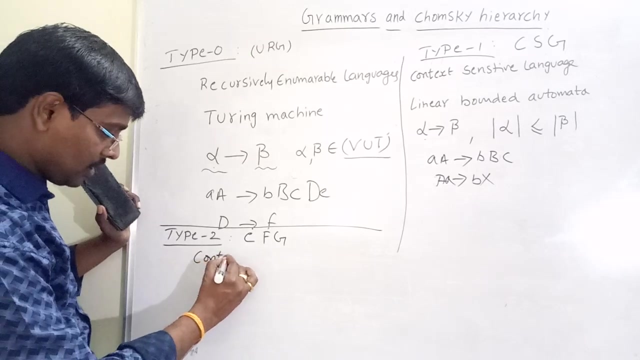 And in all the cases the left hand side is compulsory. we have to place a non-technal And type 2 grammar. Type 2 grammar, Context free grammar. Type 2 grammar is called context free grammar. The language generated by this grammar is context free language. The language generated is context free language. 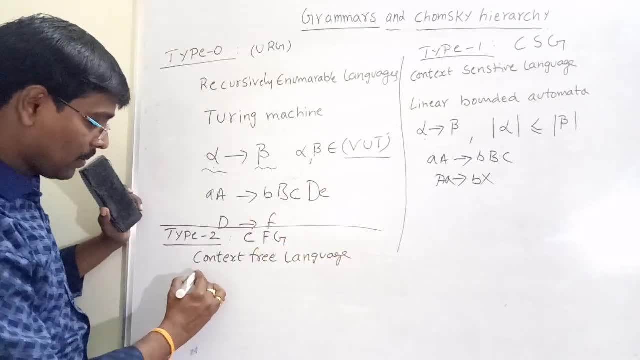 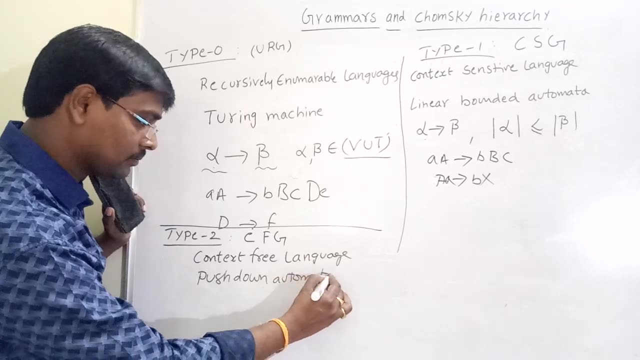 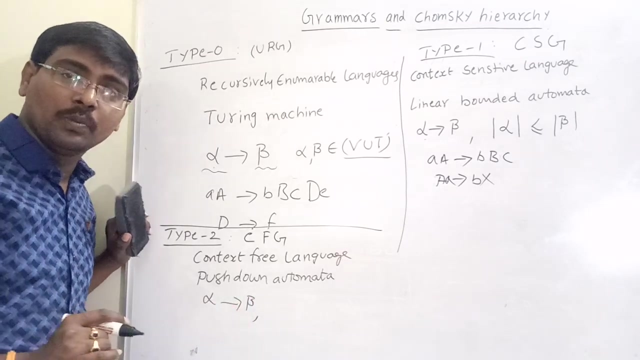 And this context, free languages are accepted by push down automata, Accepted by push down automata, Push down automata And the production is of the form: alpha tends to beta, Alpha tends to beta And always mod alpha less than or equal to mod beta. 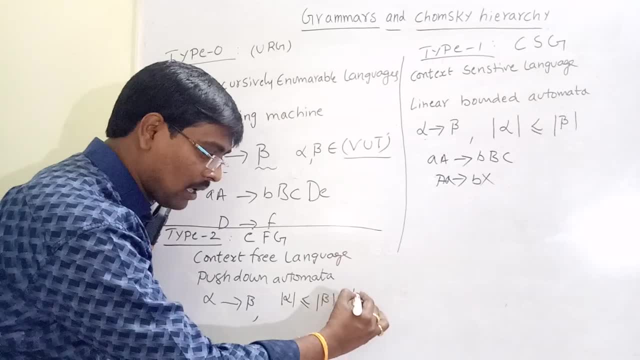 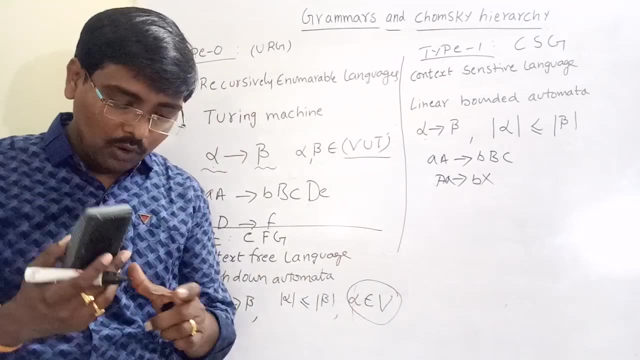 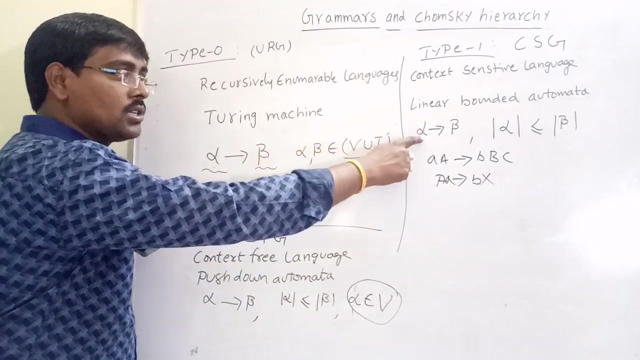 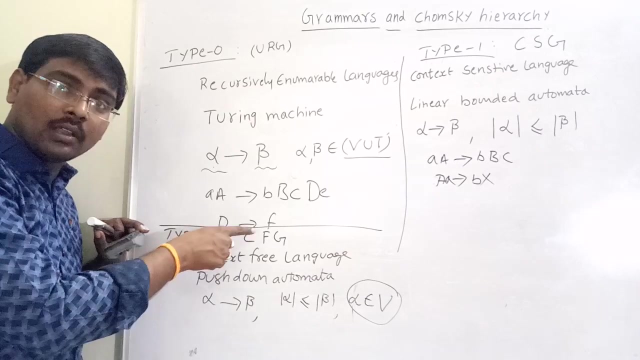 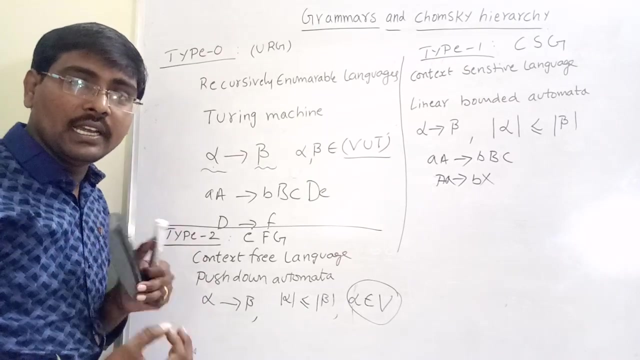 And main condition is: alpha belongs to V only. That is, the left hand side we have contains the only non-terminals. In the previous two cases, the left hand side is a combination of terminals and non-terminals, But in context, sensitive grammar. But in context- sorry, in context free grammar. The left hand side must be a non-terminal And the right side is any combination. Right side is any combinations of terminals and non-terminals. 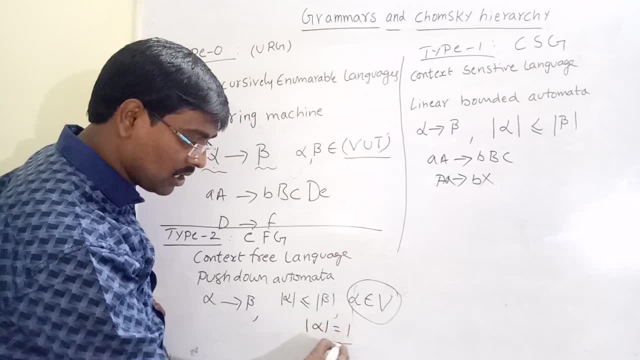 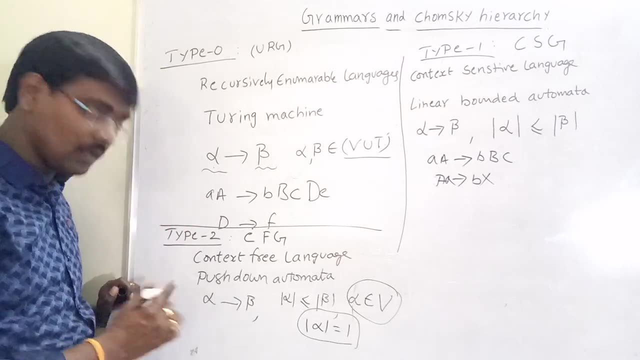 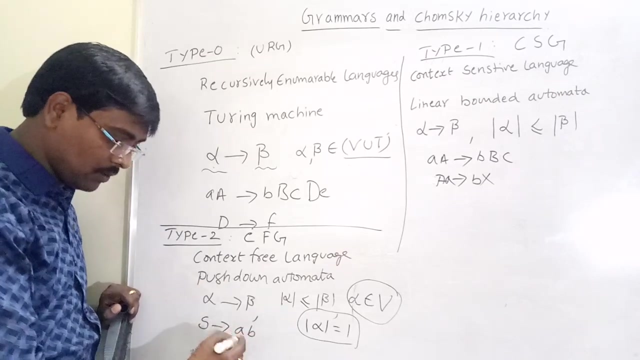 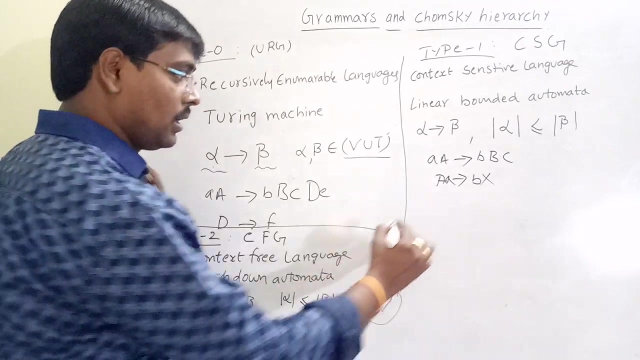 And remember mod alpha is always equal to 1.. That means we have only one non-terminal is placed on the left hand side. For example, S tends to AV A non-terminal. these are some terminals. Suppose S tends to AV A. This is also right. This is the context. free grammar And the finally type 3 grammar. 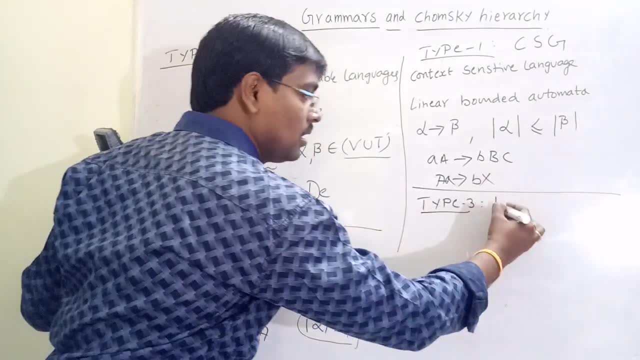 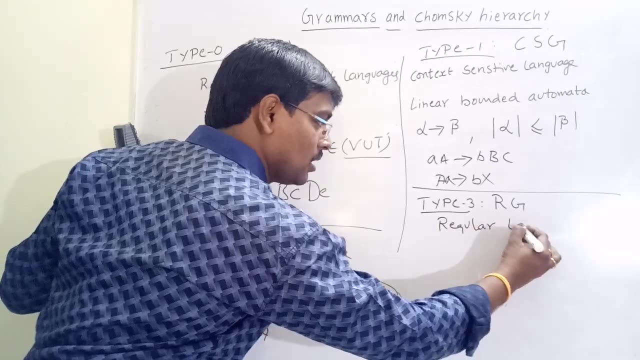 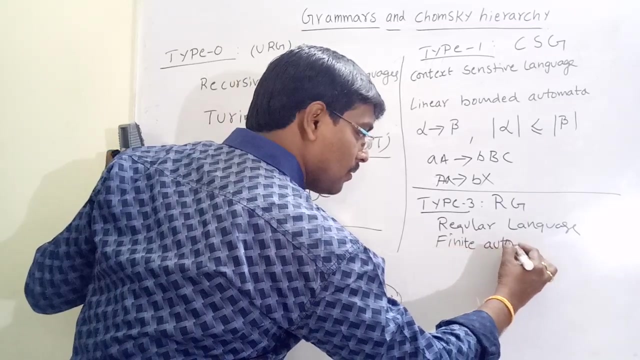 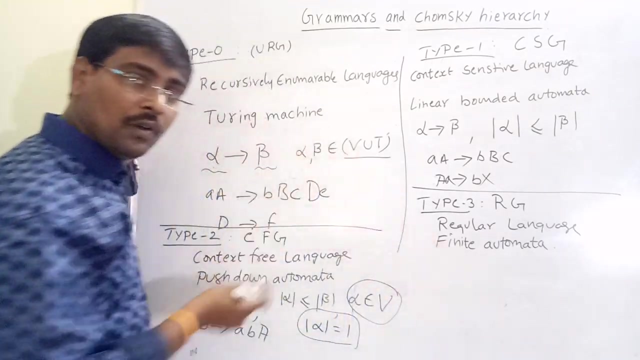 Type 3 grammar. This is called regular grammar. The grammar generates the regular languages. The languages are regular languages. It is accepted by the regular languages, are accepted by finite automata, Accepted by finite automata And the production is of the form. alpha tends to beta, Such that the left hand side 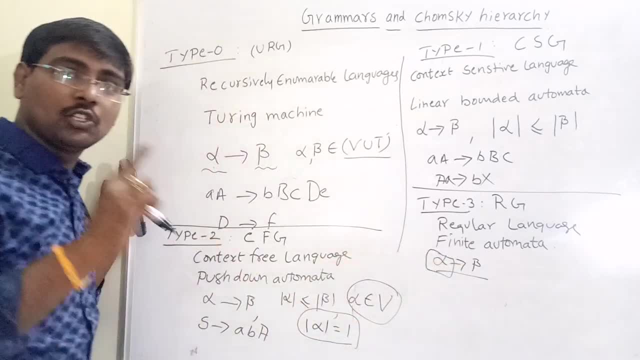 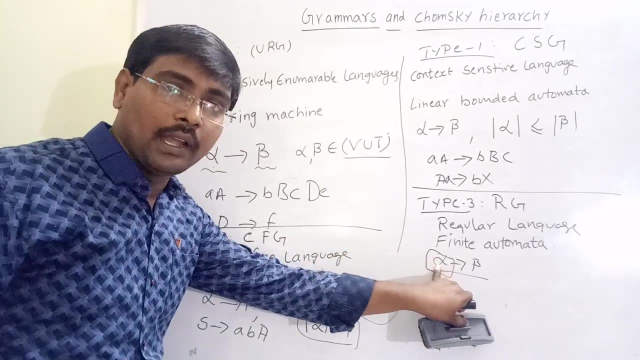 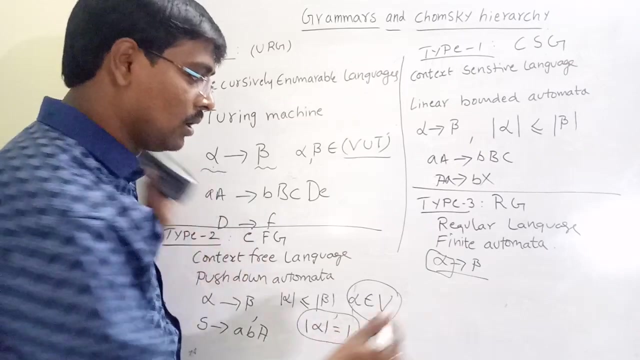 if this is the format, the left hand side must be a non-terminal, the left hand side, similar to context free. the left hand side must be a non-terminal and the length is always one that is left hand side. we have to place only one variable. for example, s tends to and the right 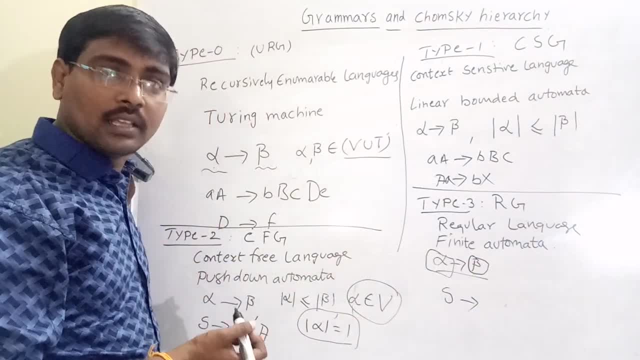 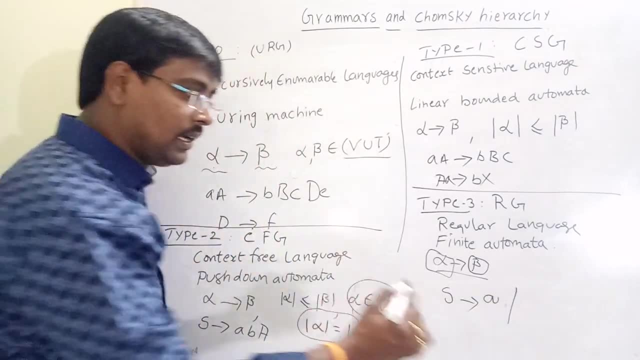 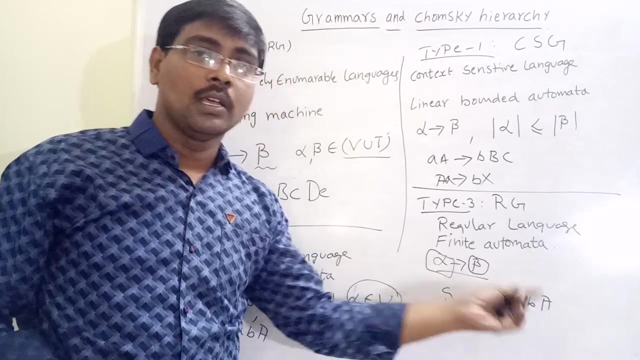 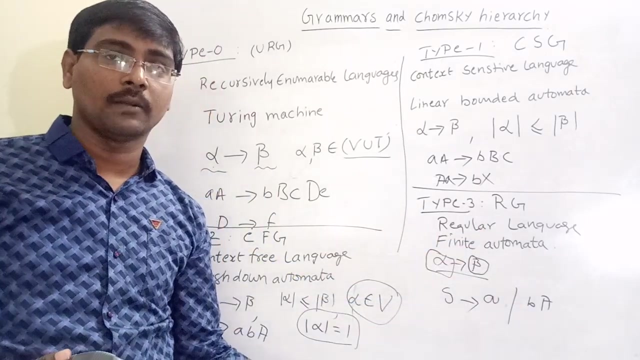 hand side is in the right hand side is a terminal, suppose a terminal, or or a terminal followed by a non-terminal, a terminal followed by a non-terminal, suppose if you are going on brief discussion, the regular dramas, we have two types, either right linear, left linear. suppose if you are using a right linear, this is the case. 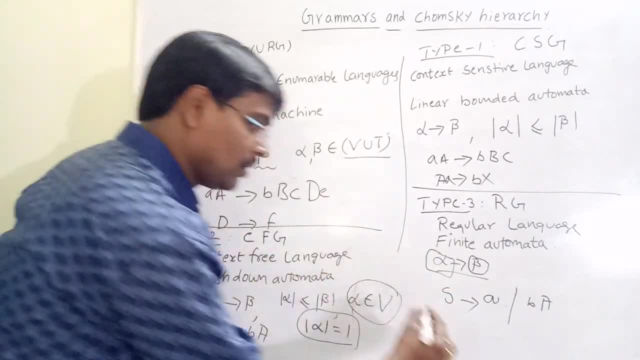 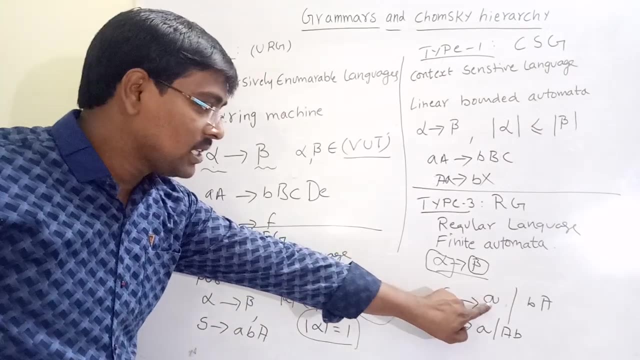 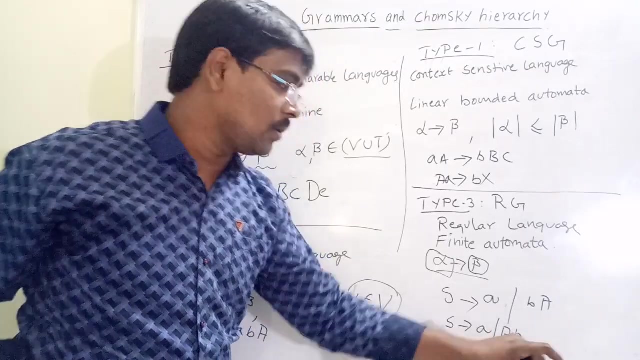 suppose, if you are using a left linear grammar, if you are using a left linear grammar, suppose s tends to AB, that is, the right side. is a terminal followed by a non terminal or a non terminal followed by a terminal, either left or right? by default we are. 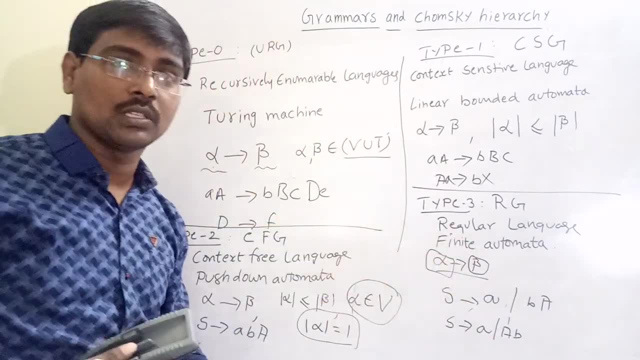 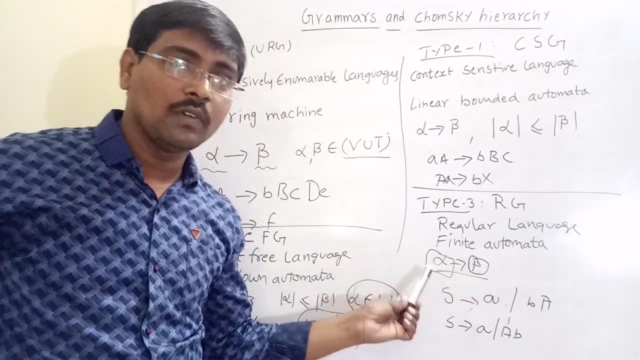 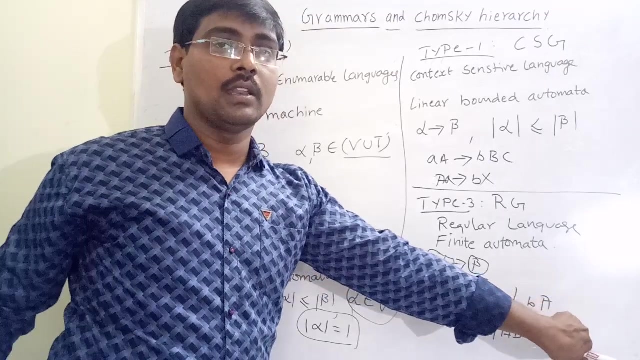 using right linear grammar. this is the rules of the grammar. so length of the alpha is always less than or equal to beta, and alpha is always a non terminal and length is only one and beta is a terminal or a terminal followed by any number of non terminals. these are the four types of grammar. 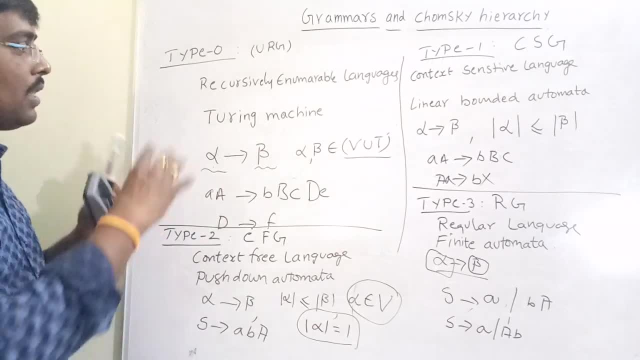 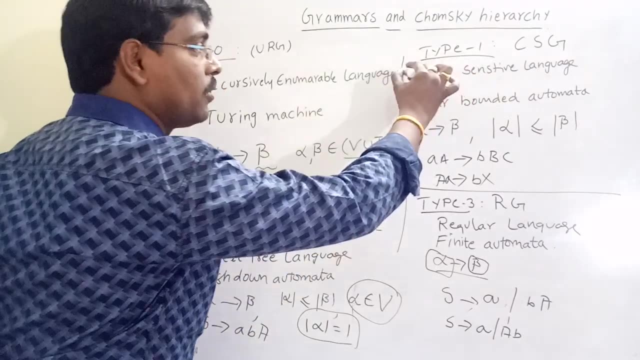 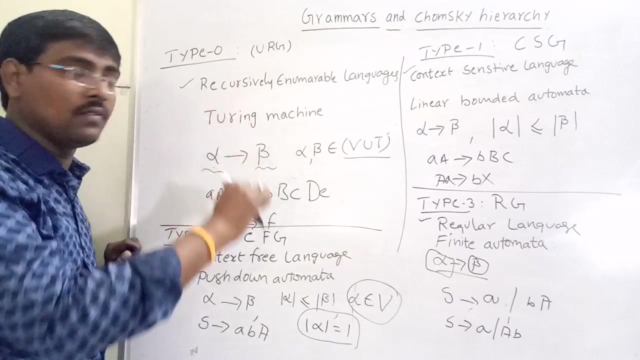 so the simple differences are: a: the languages are Type-0. the language is recursive. enumerable languages type 1: context-sensitive languages. type 2: context-free languages. regular lineways. These are the lineways: Finite automata Type 0.. Turing machine. 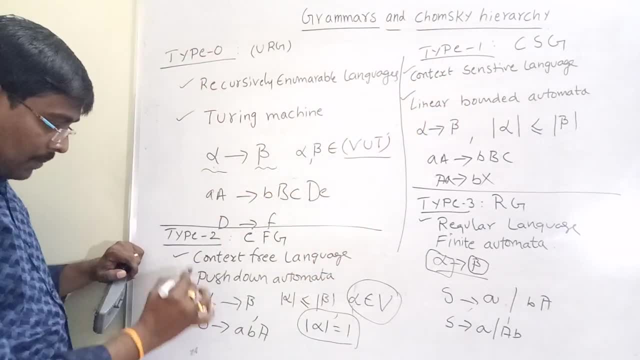 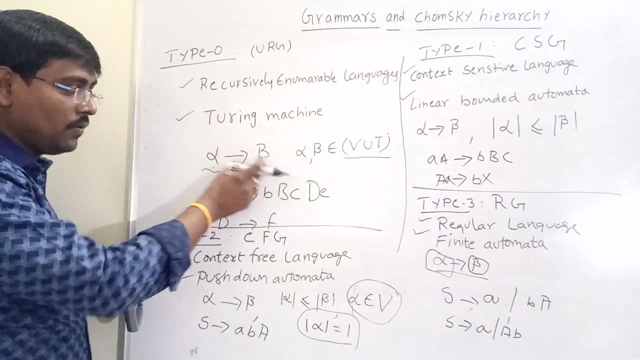 Type 1. Linear bounded automata. Type 2. Push down automata. This is finite automata. These are the production rules, Any combinations of terminals and non-terminals. Here there is no restriction. Here there is no restriction on the left hand side. 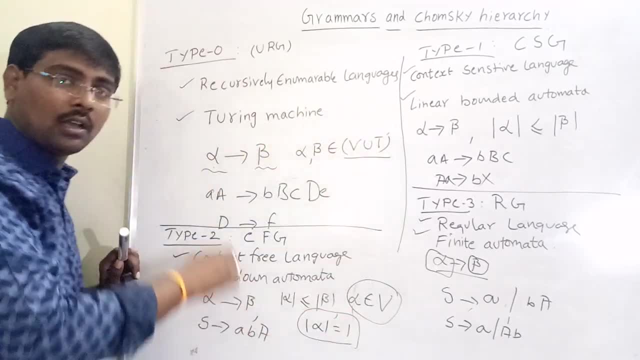 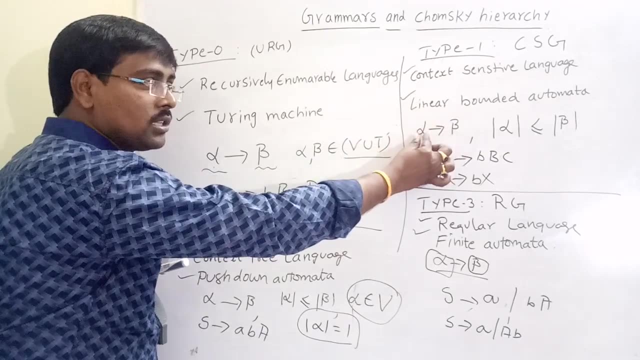 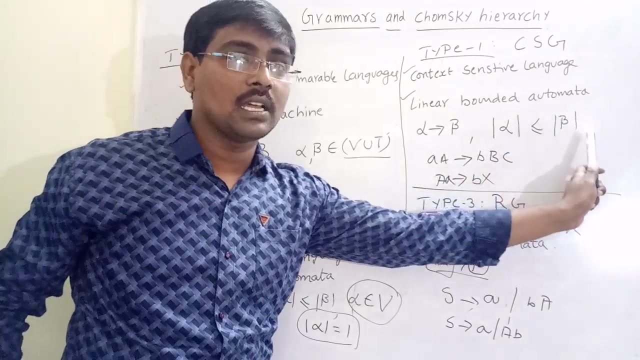 and right hand side. But remember, in all the cases at least one non-terminal must be on the left hand side. Suppose in this case here also any combination along with this one. Some additional property is the length of the left hand side less than or equal. 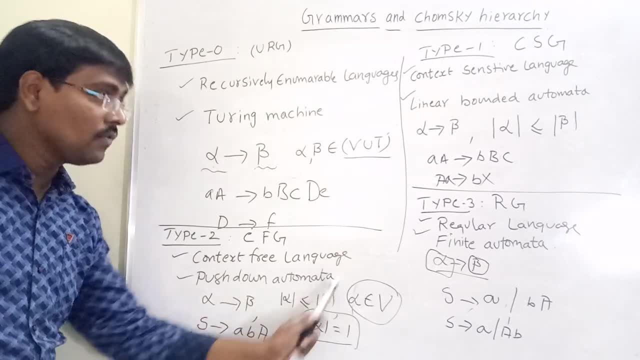 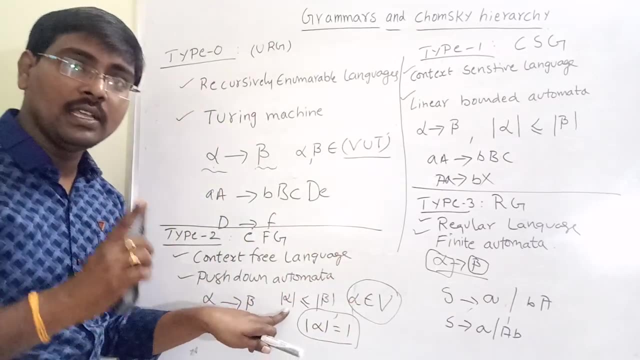 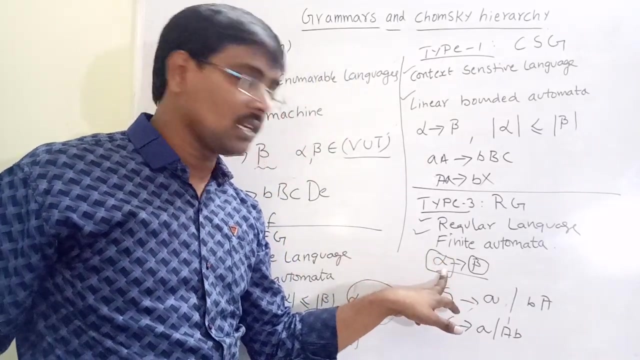 to right hand side. Come to this one Along with this property, the length of the left hand side is always 1 and it contains only a single non-terminal. Here also, the length is always 1.. Left hand side And always contains a non-terminal. 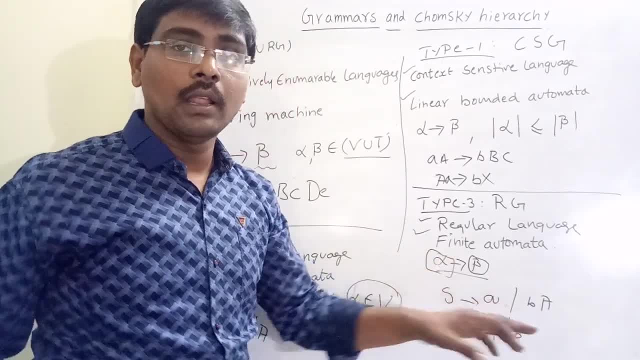 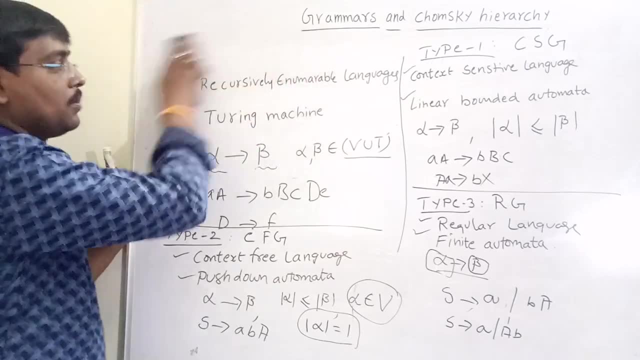 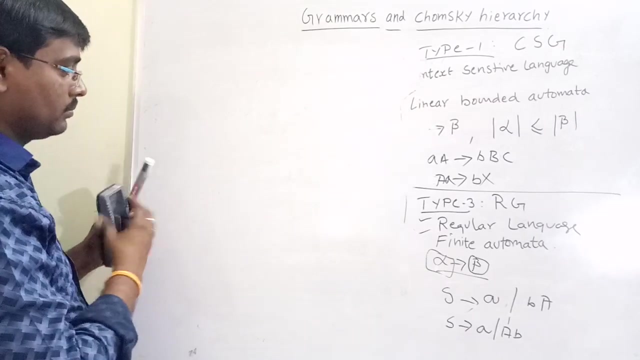 Always contains a non-terminal And right side is a terminal or a terminal followed by any number of non-terminals. This is the Chomsky hierarchy. Suppose, if you want to represent in pictorial format, Suppose: regular language, Context: free language.